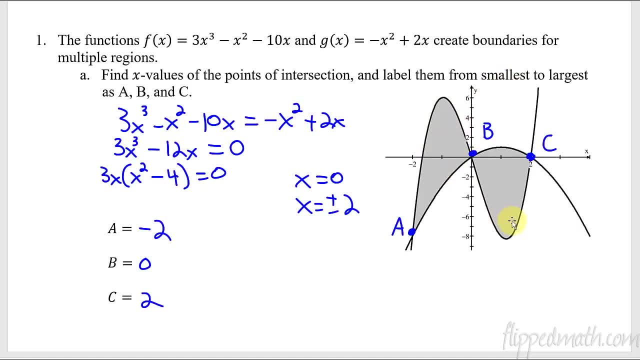 we're going to end up with two integrals because we have two shaded regions, And the reason we have to have two integrals is because the one that's on top- here the graph on top is- in this case it's the cubic, And then here the graph on top is the 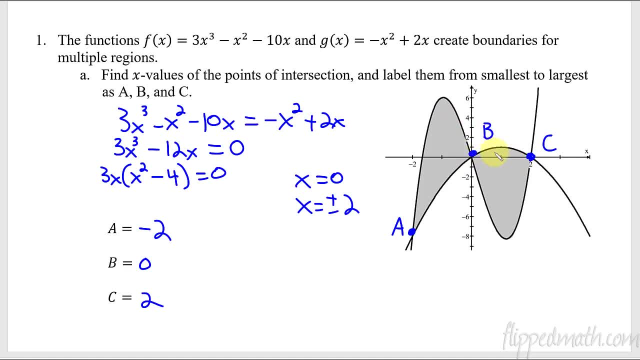 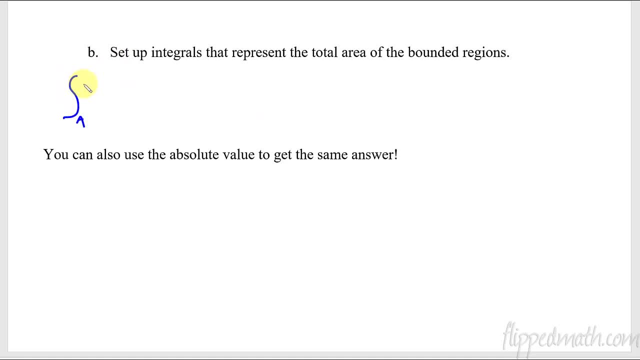 quadratic, And so it switches the functions, which one we put first. with the subtraction, We've got our first integral from, and I could say a to b, but the numbers are so simple, right? I don't? I mean, it's just a zeros and negative 2, positive 2.. Let's just put negative. 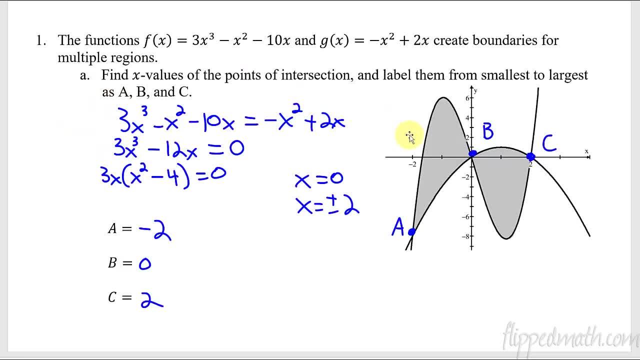 2 to 0.. Now, which one came first? It was the cubic, So let's write that out first, And then we will subtract the one that was the quadratic, which was this one: negative x squared plus 2x. 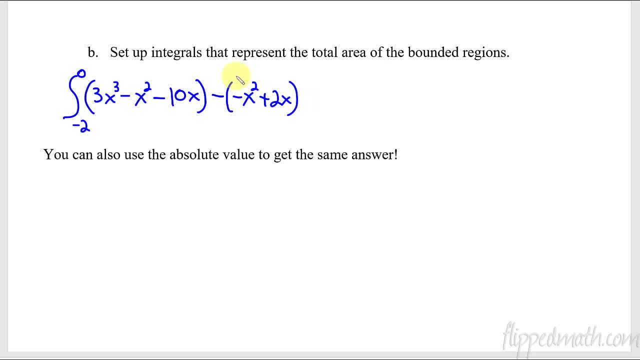 Okay, So we're going to subtract the one that was the quadratic, which was this one negative x squared plus 2x- And if you notice, I made sure that there were parentheses around this, because I am subtracting the whole thing And then I have to say that it's with respect to x. Technically, I should probably 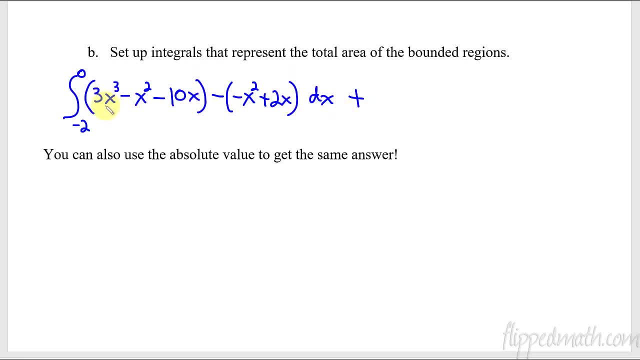 put brackets around the whole thing to make it look right that I'm it's d of x of everything. Then I go: what's my next integral? I'm going from 0 to 2.. And then now I swap them right. 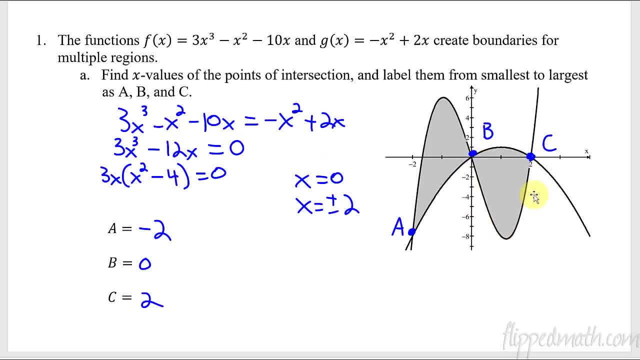 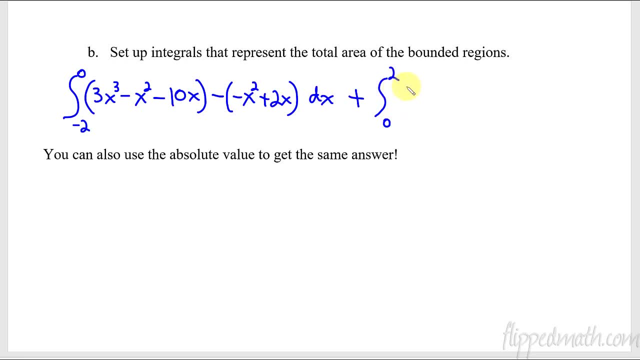 The cubic is underneath. If I look at the picture, the cubic is now underneath and the quad, the, excuse me, the, yeah, the quadratic, the quadratic there is on top. So I just switch them around and you get this here Now. I could then, uh, look and see, like, does anything? 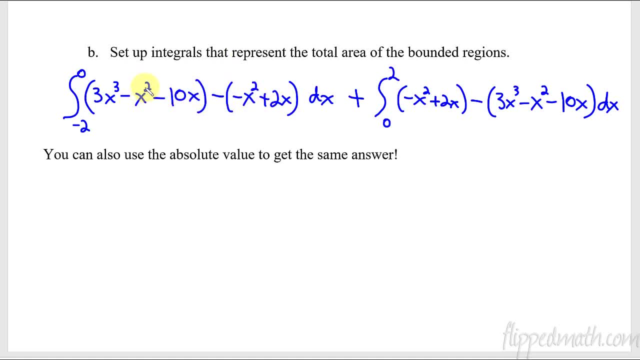 combine like terms. Yeah, If I distribute this negative, I've got x squared and an x term. they would combine. uh, same here: the x squared and the x term would combine. But for this lesson I'm just showing you how you set it up, Your answers. when you check your 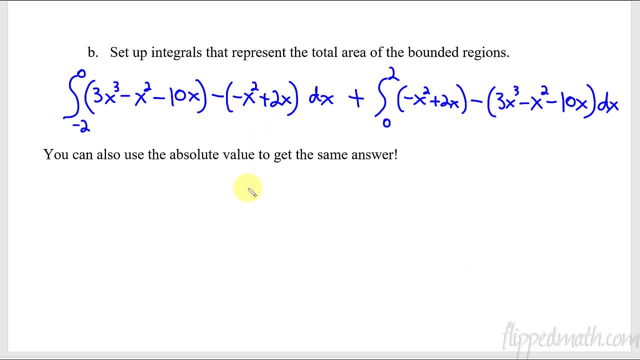 answers. for the practice, the answers will have them simplified. They'll combine like terms and put it all together, Just so be careful about that, So you know if you're doing it right. there's kind of a cool way to cheat on this, And that is if you're able to use a calculator. 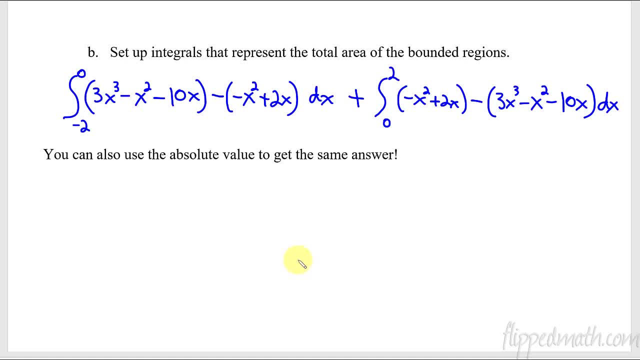 this is kind of cool. You could use an absolute value for this. Here's how that works. You take the absolute value of the difference of the two functions from a to C instead of a to B and then B to C. you just put it all. 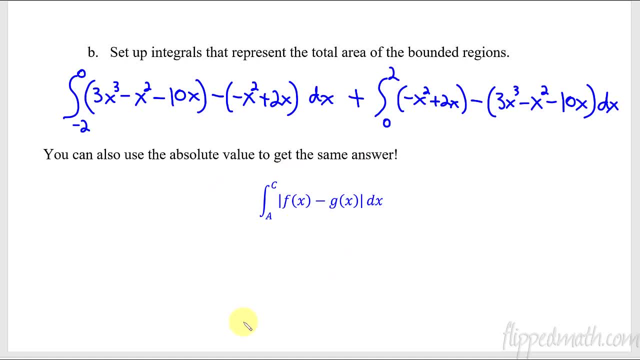 together right Pause and write this down, if you don't have it, Cause I'm going to go back to the other screen. So right here I've got my function F on top right. This one's F, this one's G. 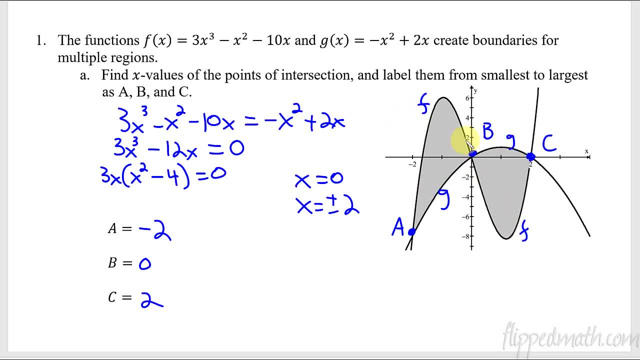 And then here G is on top and F is down there. But when you take the difference of them see here it's F minus G And then here it's F minus G. If you kept the order the same, I know this is confusing If you left it as F minus G. 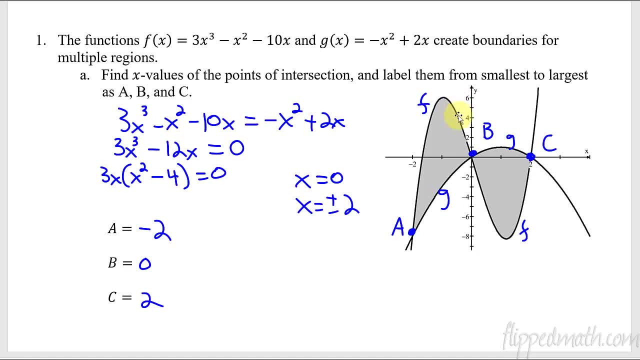 and didn't have the absolute value. and did not have the absolute value, it would be this area. And then this area would be F minus what's on top, which would create a negative area. And so by taking the absolute value, it makes it positive. Basically, it just flips these things completely. 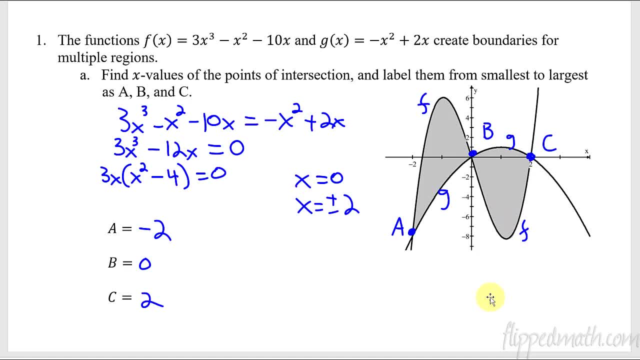 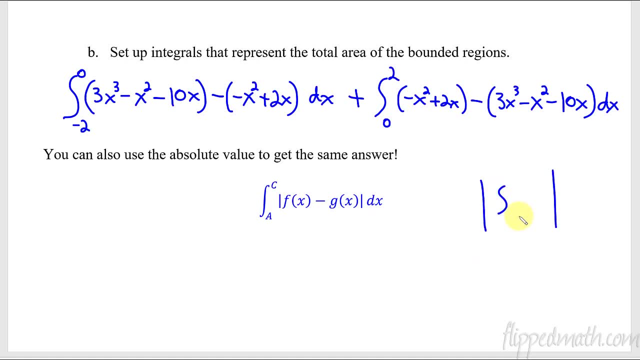 around by putting the F first. Now that you want to be careful if you ever use this, that you want to be careful that you don't don't do the absolute value of the integral like that right Of blah, blah, blah blah of D of X. 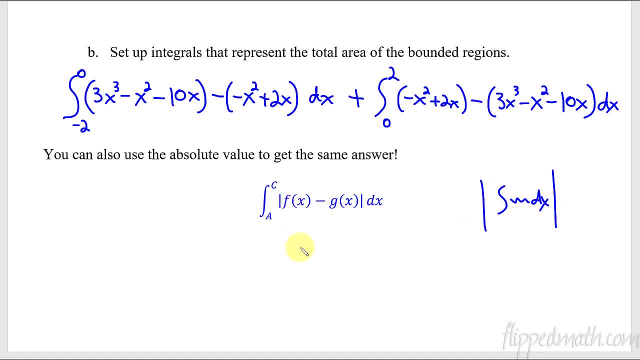 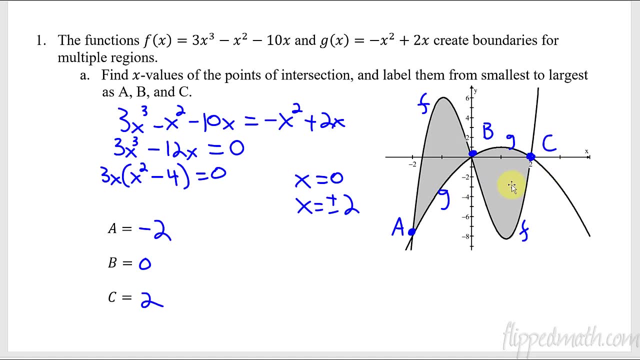 You don't want to put the absolute value on the outside. That does not give you that. But now again, that's only most students. You want to break it up and use A, B and C separately, like this, and set up the three integrals, because often you won't be allowed a calculator on these. 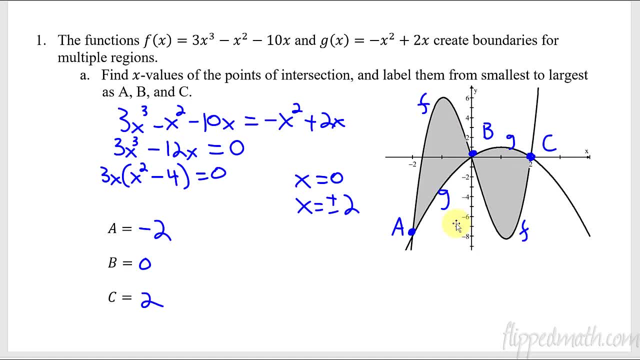 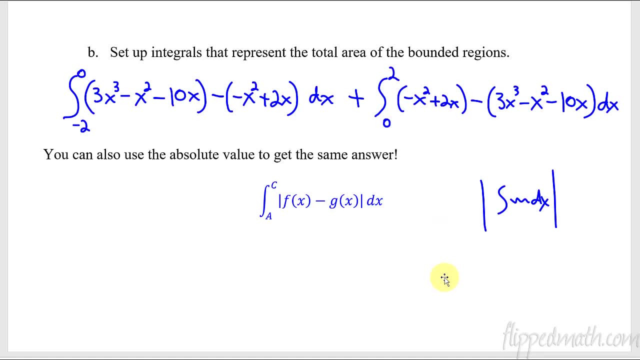 problems for this practice? you will, but I'm making you set up all of the integrals, So don't just use the absolute value on this. but I thought I'd throw it out there because I did see just a couple of test questions. 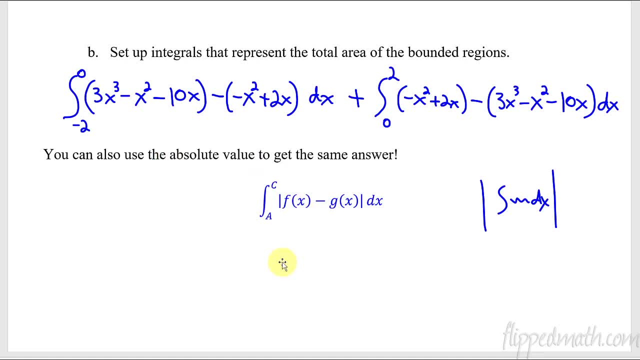 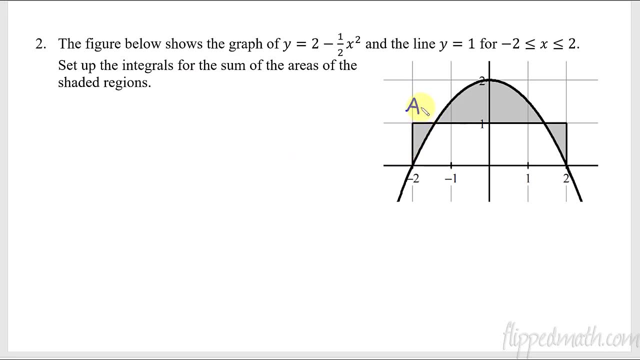 This is almost like the regression. This is my test, because this is. I was going through a whole bunch of different exams that had something like that on it. Okay, Last one. So now we're going to say: we have a, this as our a, we'll go there, and this one as our B. now notice that it doesn't cross a nice simple grid, and so you. 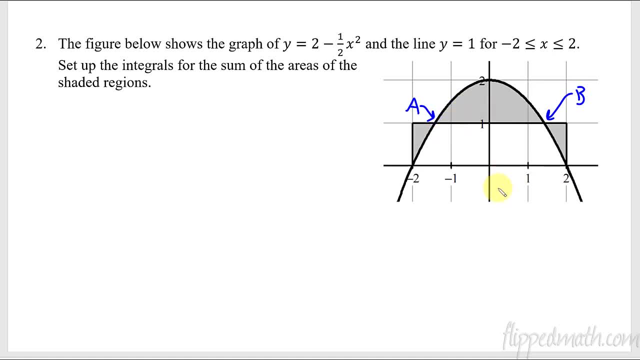 might have to use a calculator to find the point of intersection. let you know how you can store it. store a point of intersection- We've practiced that in our last lessons- And then you can set up your integrals with an A and a B. This one happens to be easy enough because there's only this one variable. 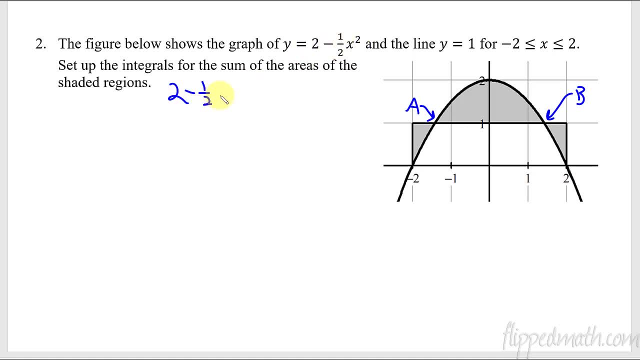 right there that we could solve it without needing the calculator. let me show you how you do that. you just take this and set it equal to each other. this, you have this one, you set it equal to one, the other line- and then you can solve from here. multiply both sides by negative 1 half, and then you take the. 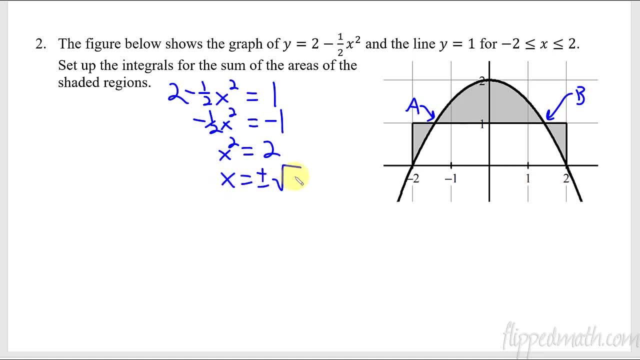 square root of both sides, you end up with plus or minus the square root of 2, so this one's the negative square root of 2, this one's positive square root, 2. and now that lets us set up our integrals. now, how many integrals will we need? 1, 2. 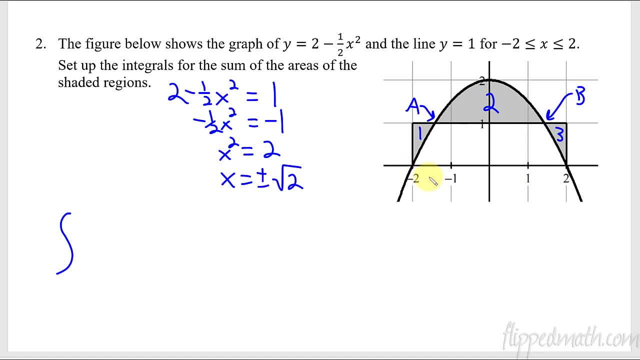 3. there are three regions, so we'll need three integrals. so the first one just goes from negative 2 to negative square root of 2, so that's my a, my negative square root of 2, and if you had used a calculator you'd give me a long crazy. 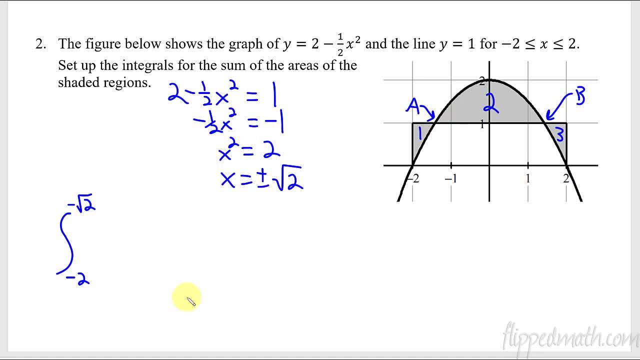 decimal and you'd have to store it as a and then you can just write a right there and then which one comes first. we've got the line that goes first, so it's gonna be 1 minus, and then the parabola, the quadratic. so I'm going to 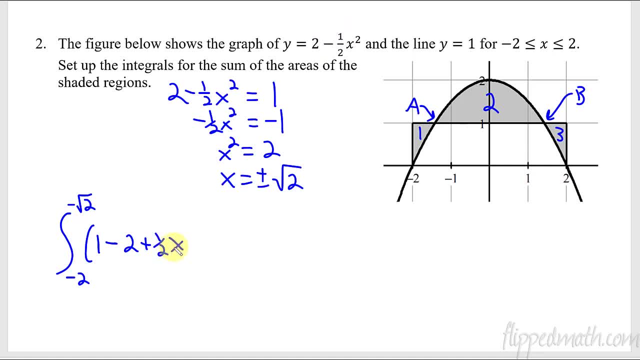 subtract 2 and add 1 half x squared. okay. so I'm going to subtract 2 and add 1 half x squared, okay. so I'm going to. hopefully you're following why I added, because I'm subtracting this whole thing, so the minus distribute distributes, and then that's with respect to X and then. 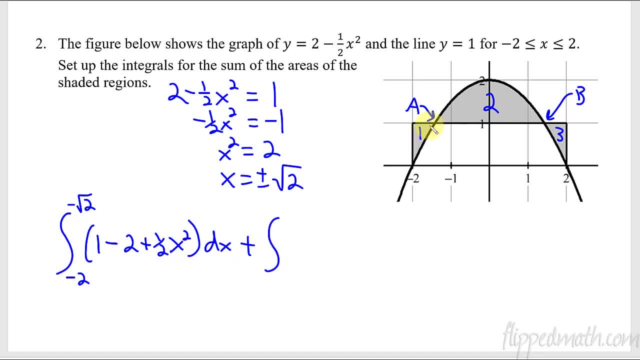 plus. so we've got region 1 down. now I do the next one. I'm gonna go from negative square root of 2 and positive square root of 2, right, because I'm doing this region, so a to B, and then now the parabola is first, so I can write up 2. 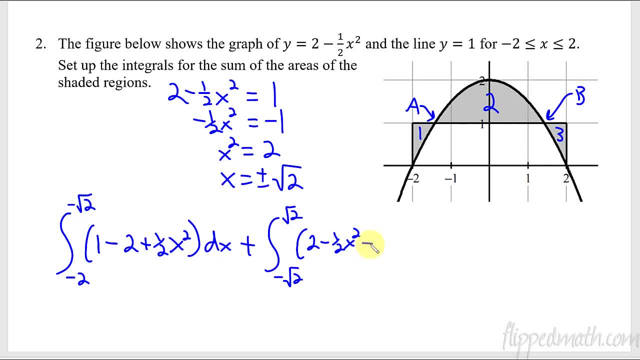 minus 1, half x squared, and then minus the line there which is just a 1 with respect to X, and then my last region. I'll have my square root of 2 and I go up till I get to 2, and which one's first. the line is first so 1 minus, and then I. 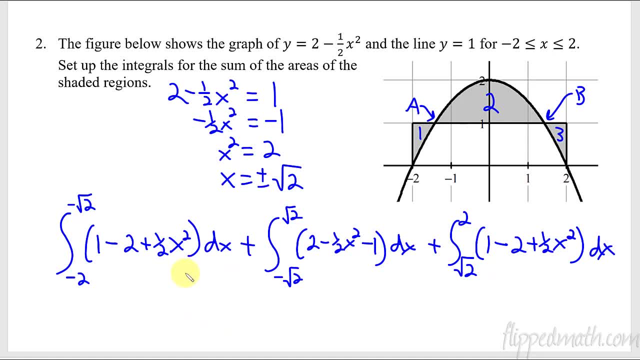 do the same thing that I just had right there. now that's the setup. I could clean this up: simplify, combine like terms: 1 minus 2 would combine, and so forth. you got all these little numbers here- constant, set combined. but this is the setup that you could then plug in a calculator to get the whole thing. 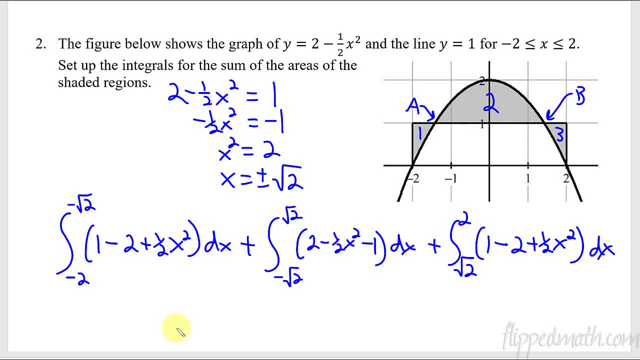 figured out okay, so that is the practice of what you're doing in today's lesson and in today's practice problems those of you who have a test up next. Good luck on that test, And then, when we come back to our next lesson, we will start getting into. 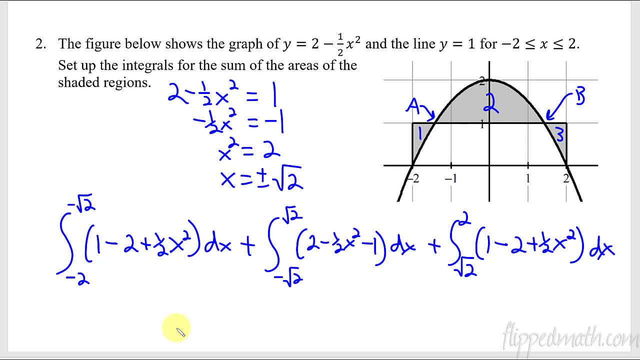 volume. We've covered everything with area now and then we'll start getting into some volume, And that's the last thing we'll have to work on this year is solids based on different graphs. It's kind of cool, It's weird stuff, but I but it's kind of cool And it's the last thing we got. 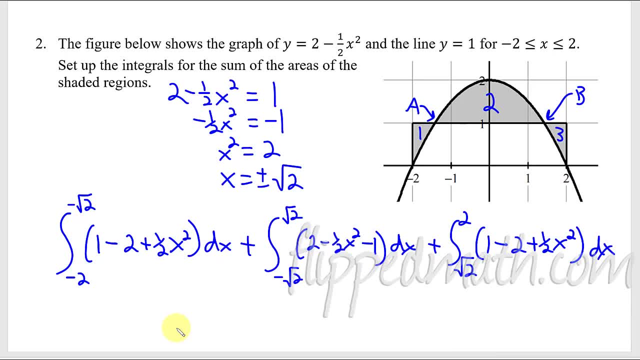 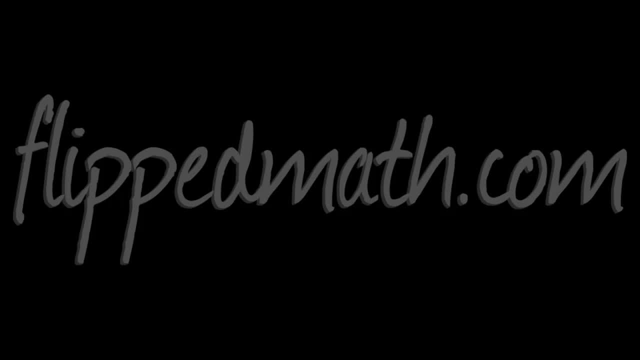 to deal with for the AB students. Okay, Rock that, master check. I'll see you back in the next one. 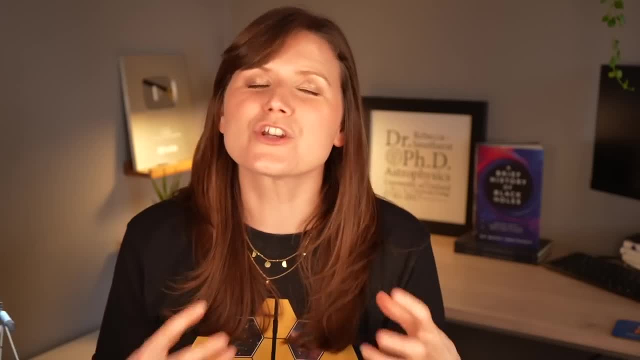 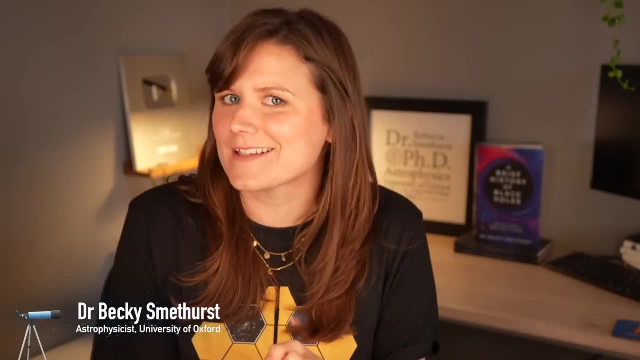 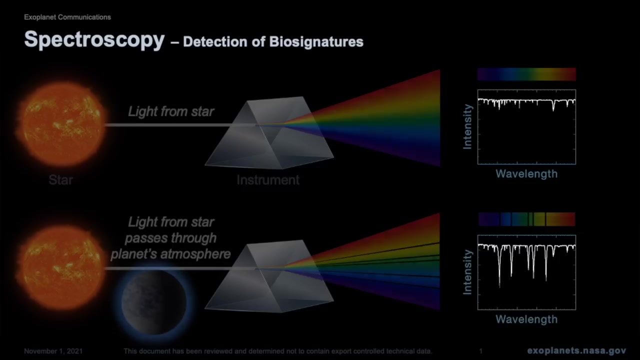 The James Webb Space Telescope was always set to revolutionise our understanding of exoplanets, planets in orbit around other stars, in our galaxy, the Milky Way- And, in particular, it was designed to collect the tiny amount of starlight that passes through an exoplanet's. 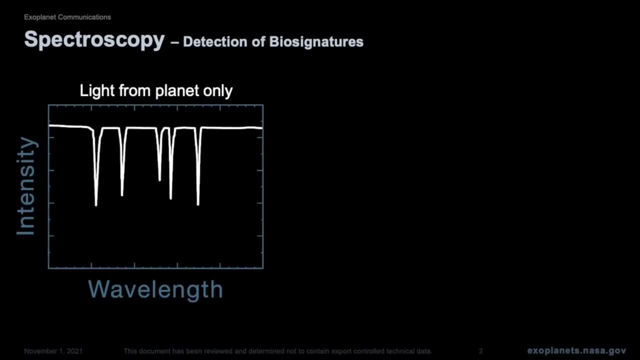 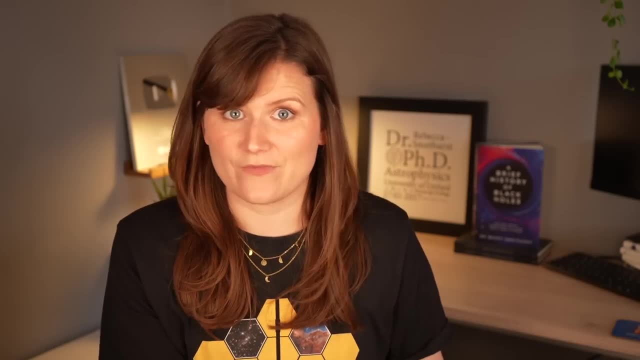 atmosphere on its way to us, so that we can work out what the atmosphere is made of. Now this is easier to do the bigger the planet and the thicker its atmosphere, which is exactly what people started with. They were learning how to do this with Jade Whisty, with planets that were the 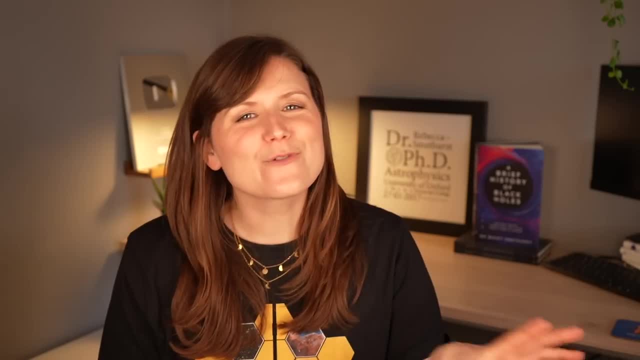 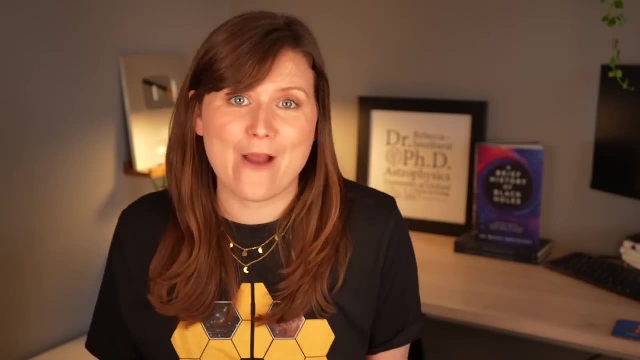 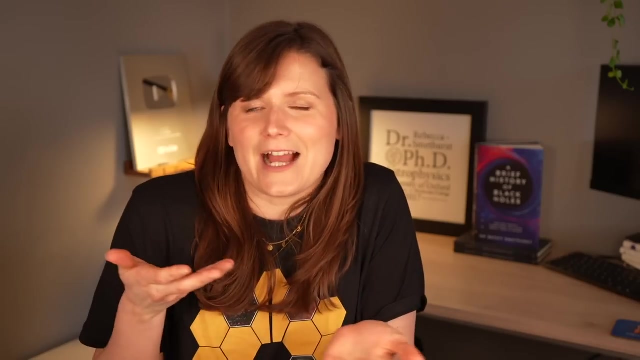 size of Jupiter or Neptune. But we all know that the dream is to do this with rocky planets that are Earth-like, that are also in the habitable zone around their star, the region where it's not too hot and not too cold for life to flourish. But to do that, we have to find them first, which is 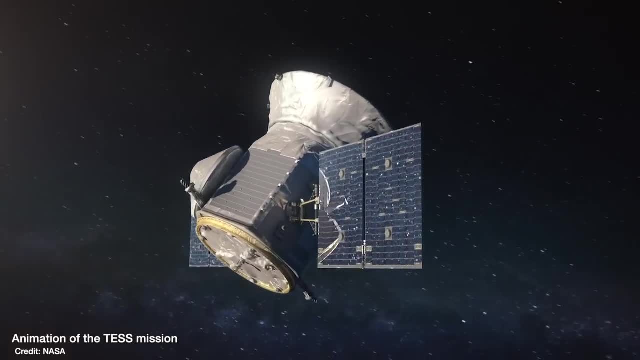 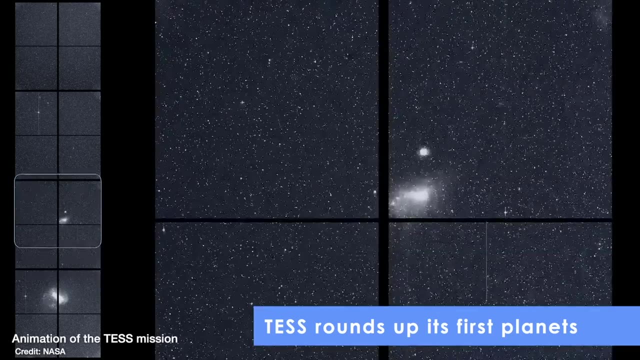 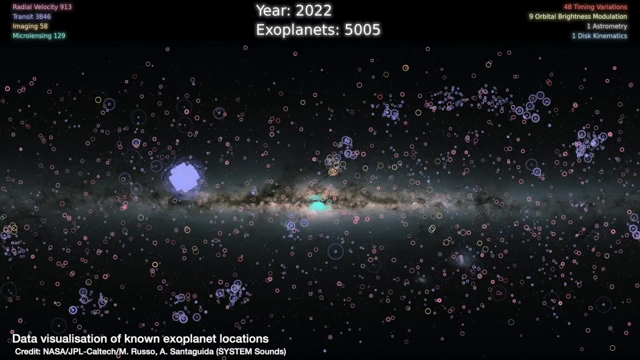 where the TESS mission comes in, the Transiting Exoplanet Survey Satellite whose sole job is to hunt for new exoplanets. Now, thanks to the TESS mission and its predecessor, Kepler, we've just passed the milestone of 5,000 confirmed exoplanets. But the majority of those are the big planets that are easier to spot and the smaller ones that we do find aren't guaranteed to be in the habitable zone. So of those 5,000 exoplanets that we know of, only 60 of them are thought to be both in the habitable zone and small enough. 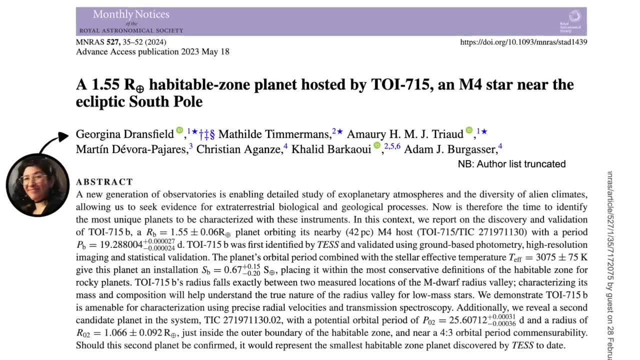 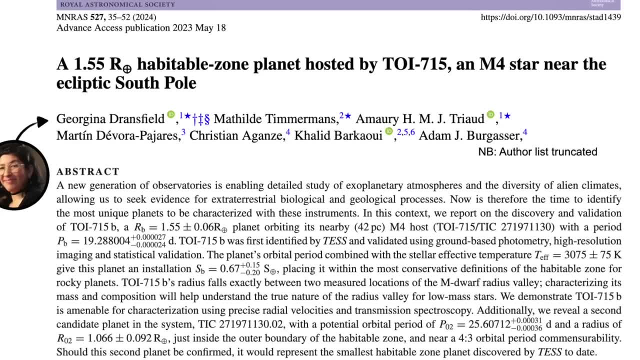 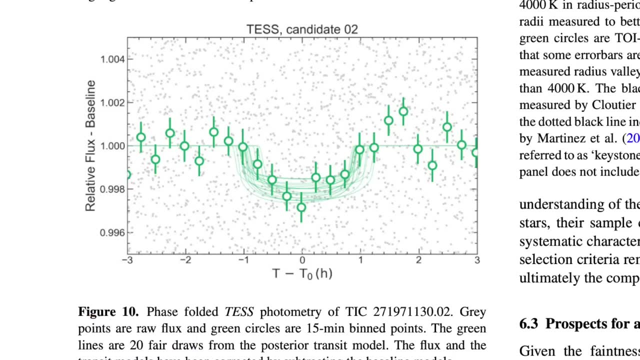 to be rocky Earth-like planets, Which is why there was a lot of excitement this past month when this paper by Dransfield and collaborators was released, announcing the discovery of not one, but two rocky exoplanets in the habitable zone around their star. Now the first one. 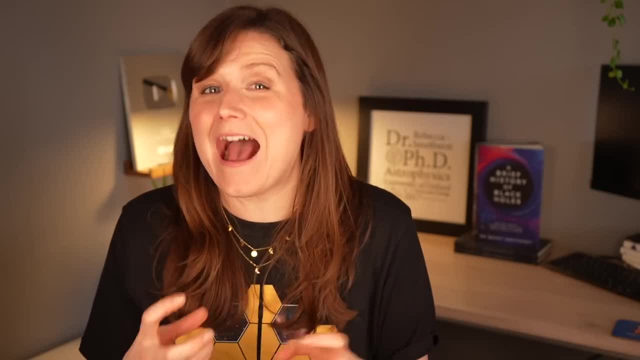 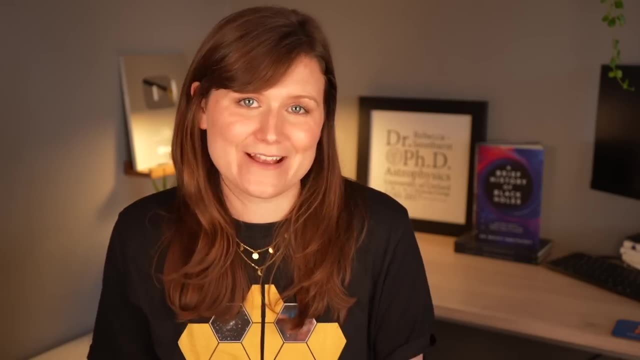 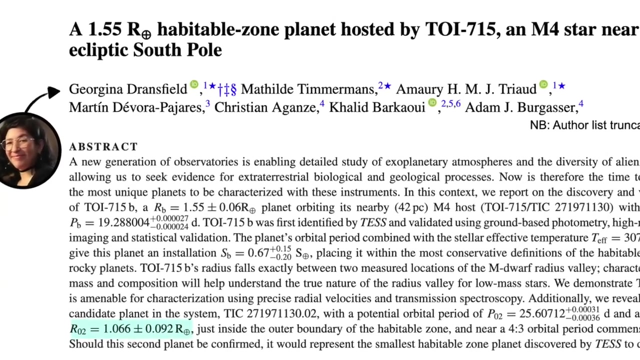 they're really sure of the detection, but the second one they're not as sure. But if it is confirmed, with more follow-up observations, it would be the smallest habitable zone exoplanet found by TESS to date, at just 6% larger than the Earth. So before we dive into all of the